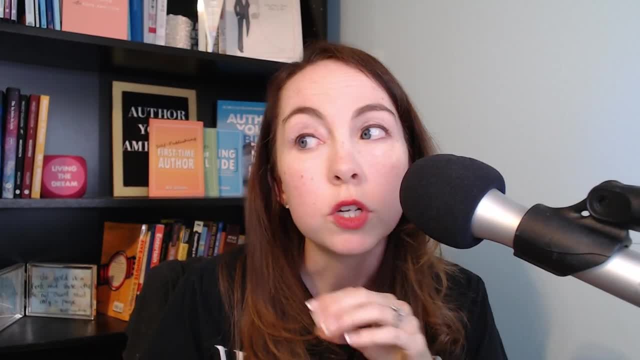 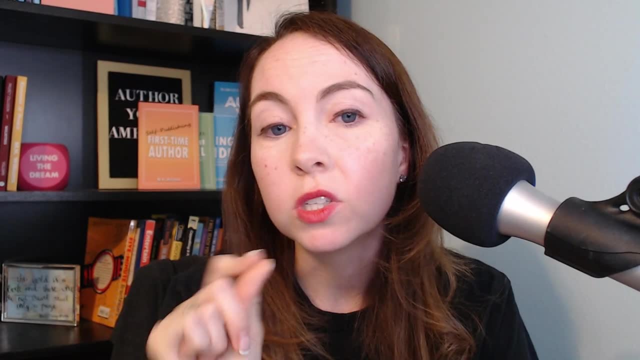 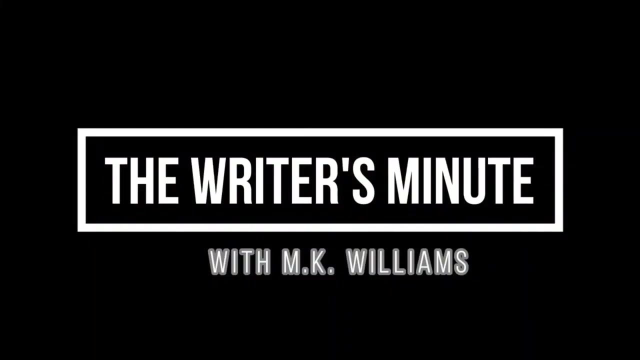 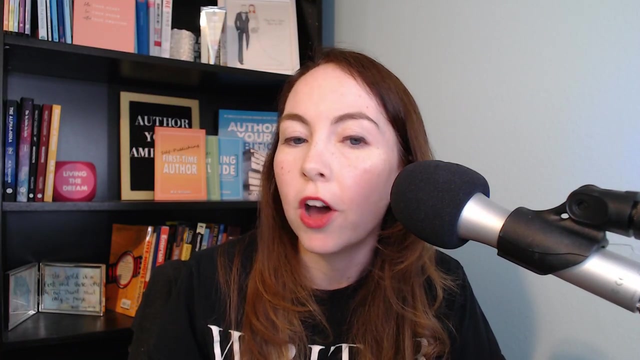 So my book is 300 pages, So it's 300 pieces of paper. Do I say it's 300 pages? when I upload it It's a page, but it's both sides, So it's two pages. Hi, I'm MK Williams. I'm an author and independent publisher. I love sharing my insights about all. 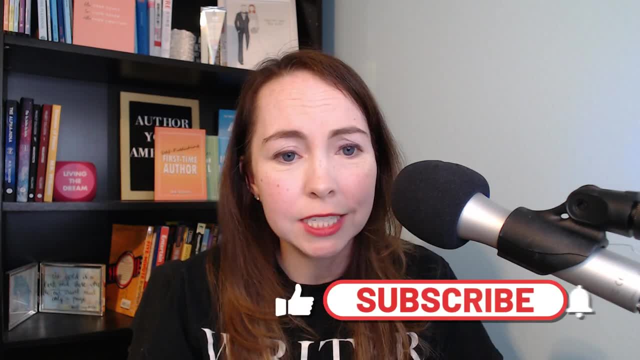 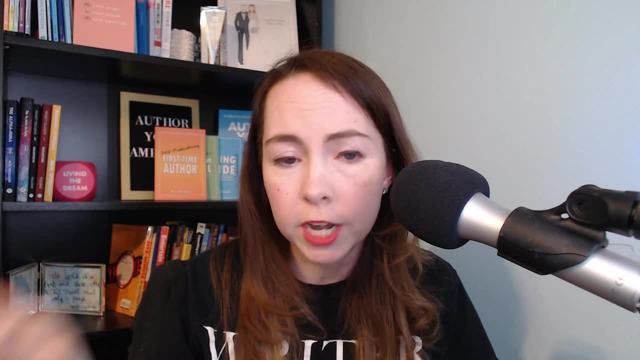 things- books and publishing with you. Before I get into the details about today's topic, don't forget to hit subscribe. You'll be notified when I put out new videos every week about publishing, making a career being an author and now being an entrepreneur. So this is going to be. 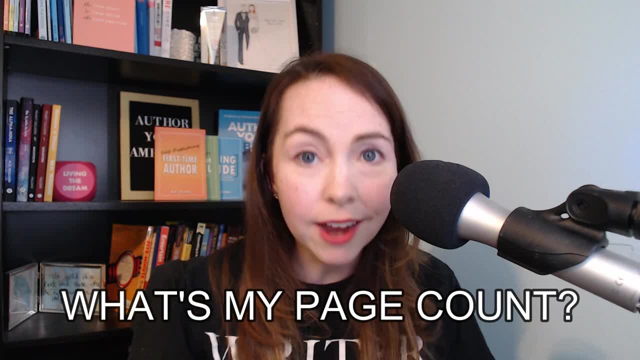 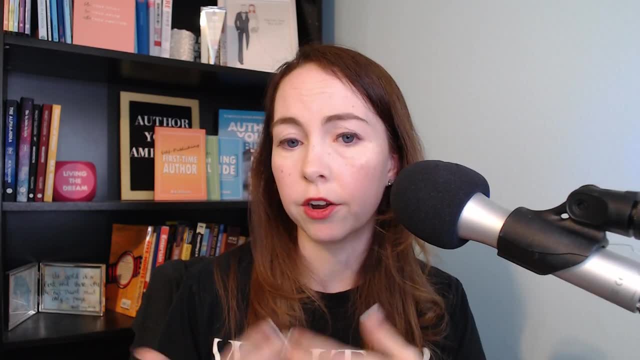 a short and sweet video, but I've seen some questions on this exact topic so I wanted to address it. When you are talking about the length of your book, you have a few ways to do it. When I'm talking with an editor or formatter, they usually like to know the word count of the book. 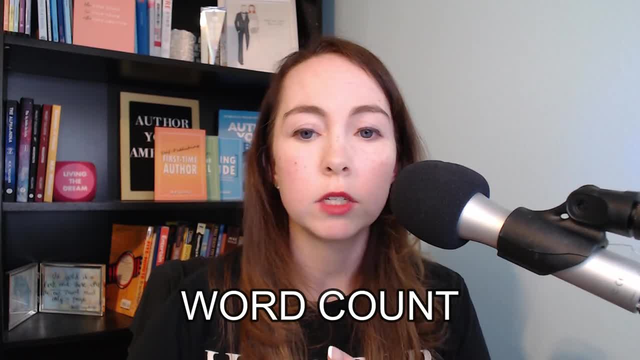 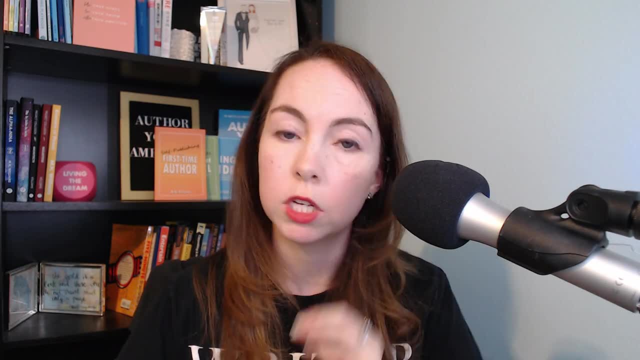 because, regardless of the font size and line spacing, the word count tells them the length of the book in terms of how much they will have to read When it comes time to upload the book, or tell your cover designer the page count so they know how big to make the spine. they need to know the number of pages. 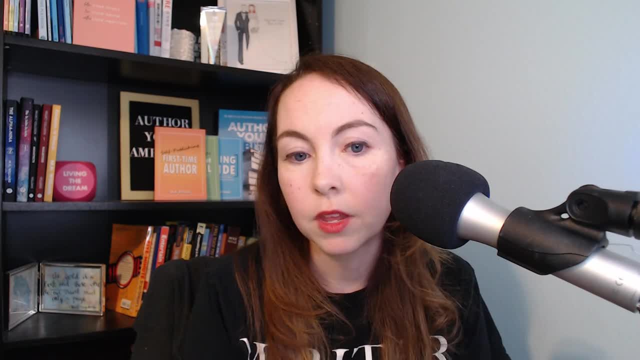 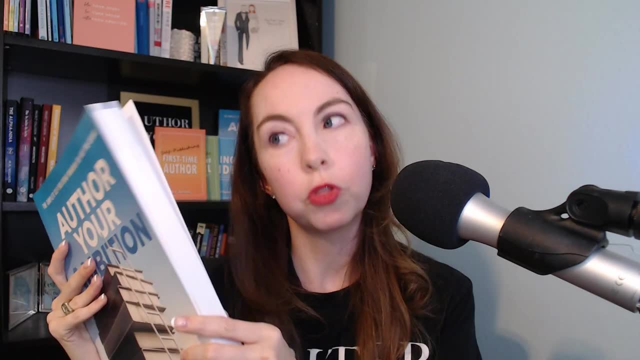 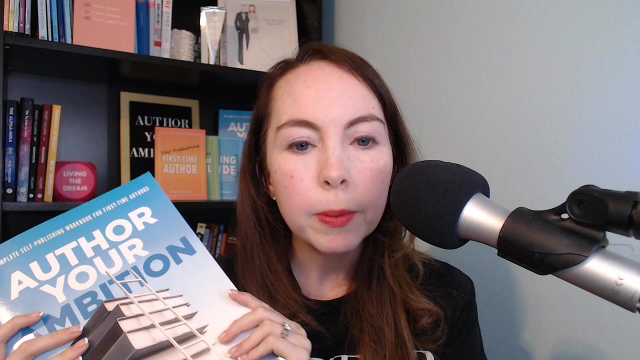 So is it a page a page or is it a sheet of paper? Best to use an example. So let's say I have a final formatted page count for a book that is 300 pages, as in. you open the PDF file and it says one out of 300 pages. Now you probably have like 290 pages of actual book. 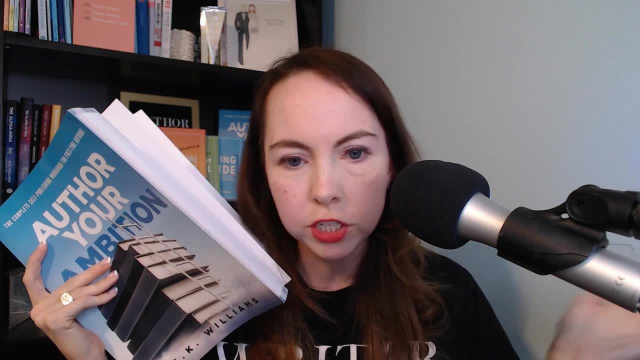 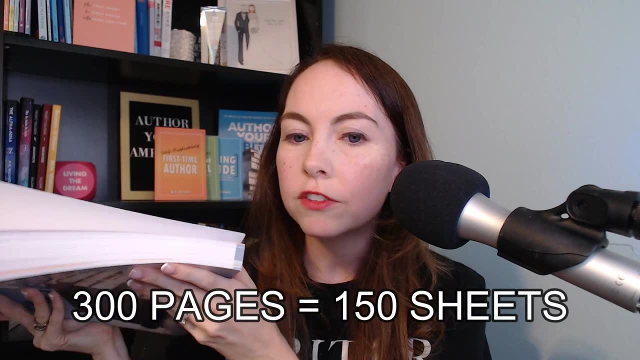 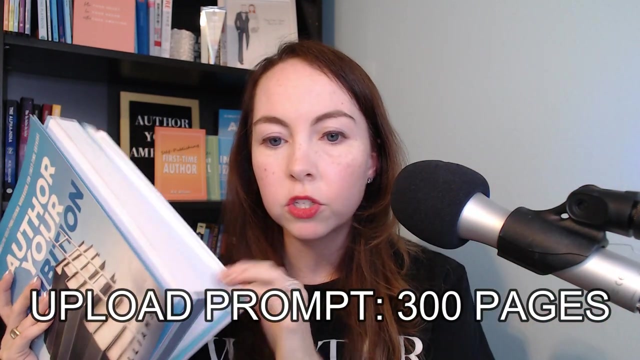 And maybe 10 for the dedication, table of contents, copyright, page acknowledgements etc. But the all-in page count is 300 pages. So the book will contain 150 sheets of paper printed on both sides. The sheet refers to the actual leaf of paper. The page count is the total number of. 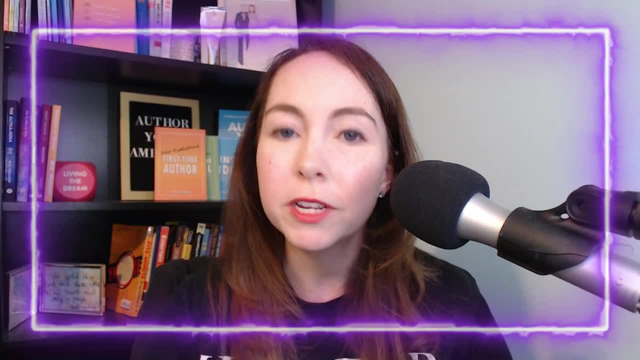 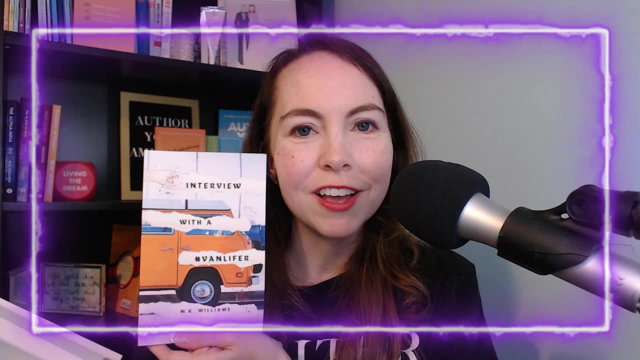 printed pages, And this video is brought to you by two of my books. The one with the largest page count, my Author, Your Ambition workbook, and the shortest page count my Hippie Vampire Novella. Interview with a Vanlifer. 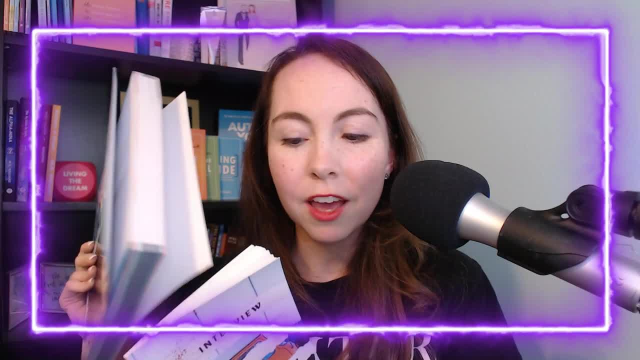 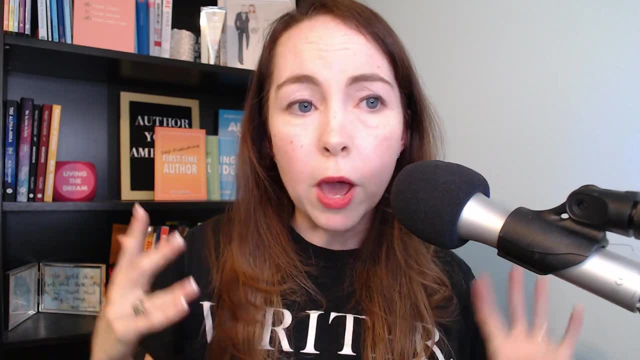 That's right. Books come in all shapes and sizes, but each of them have pages and multiple sheets of paper. All right. What other super niche-y, minutiae questions do you have about publishing your book? Let me know in the comments below. That's literally all I do here is answer these.